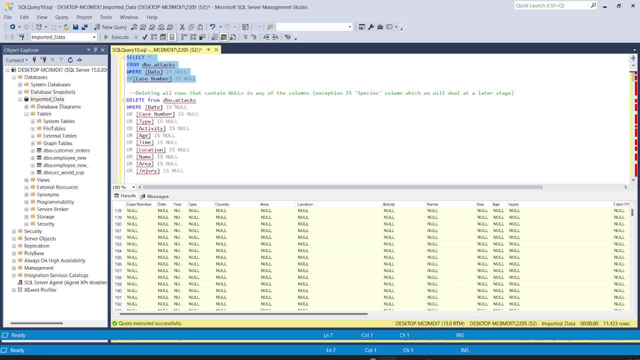 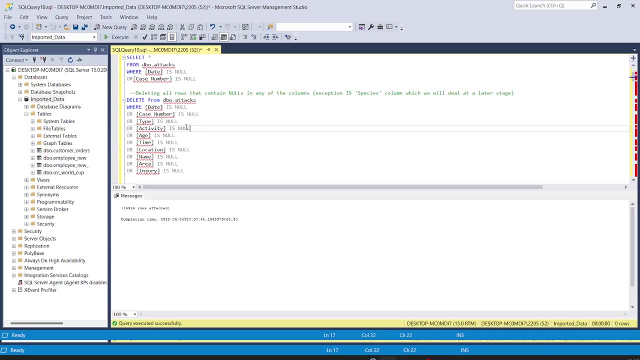 So for that we will write this command: delete from the table name where our date is null and these columns are null. So let's run this query. So now you can see 14,324 rows are affected. So it has deleted all the rows where these columns were null. 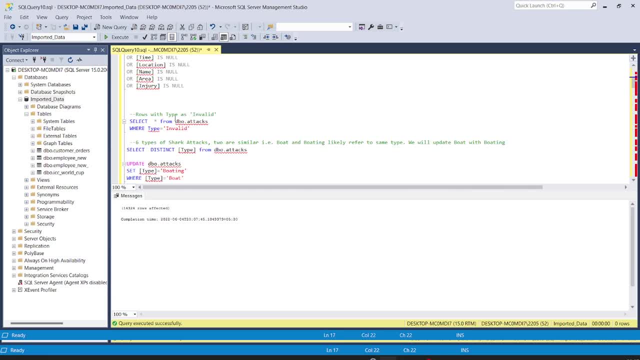 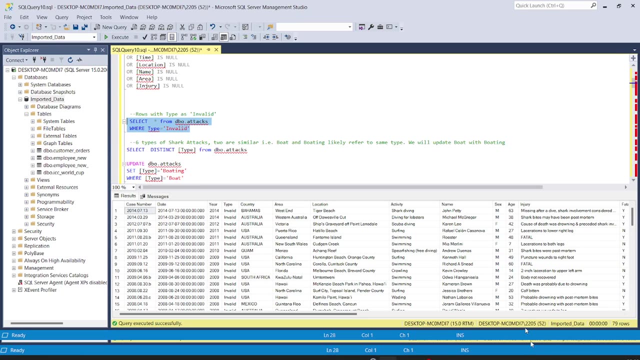 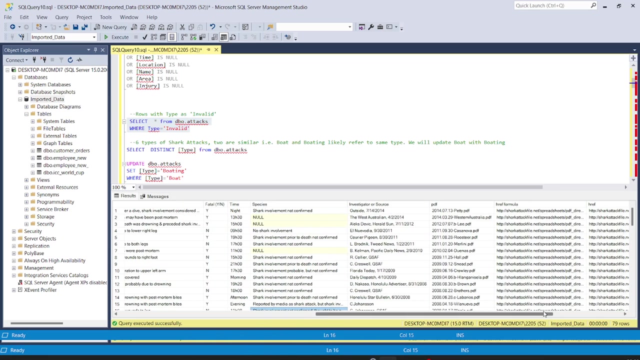 Okay, So now we need to find rows with type as invalid in our data set. So for that we will write this command: select from attack table where type is equal to invalid. So let's run this code. So now we have total 79 rows where type is invalid. 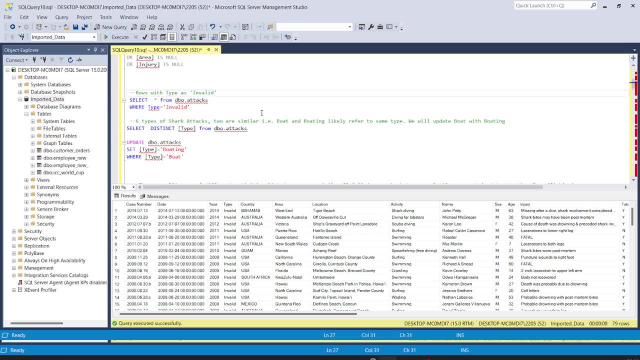 So, as you can see, that type is equal to invalid. So now let's check how many types we have in this type column. So for that we will use distinct. So select distinct type from attack table. Okay, we will run this. 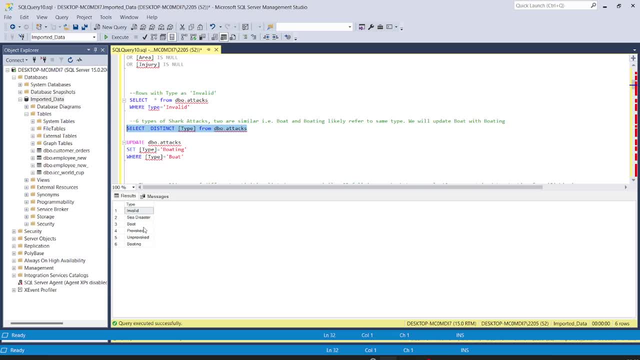 So we have six types here and two are similar. As you can see, the row number three and row number six- vote and voting likely refer to same type, So we will update this vote with voting. Okay, So for that command is update table name, which is attacks. 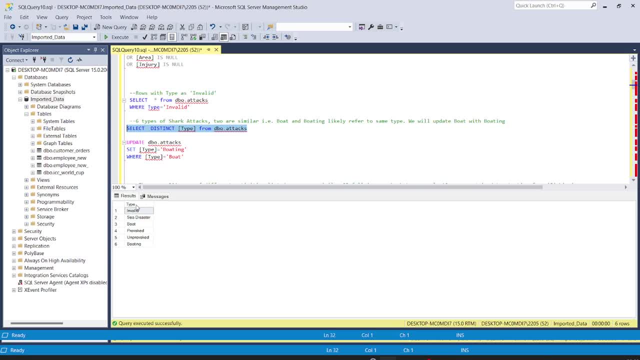 And we need to change the value of this type column. So we need to set: type is equal to voting, where type is equal to vote, Okay, we will run this code. So seven rows are affected. So in this whole data set we have seven rows where we have vote instead of voting. 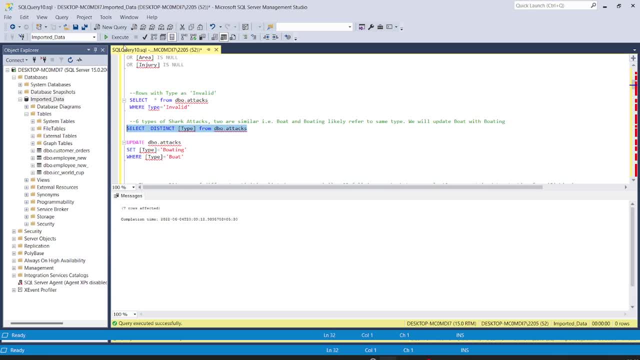 So let's run this query again: Select distinct type from debut. So now you can see we have only five type. Okay, After that, same thing we will do for activity as well. So in order to know that total number of activity in our table, we will write: select distinct activity from attacks table. 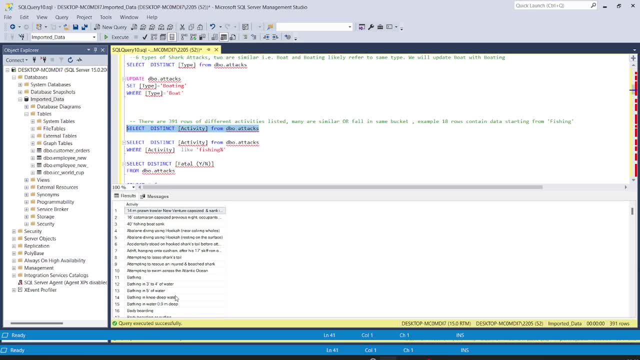 So we have total 391 rows- Okay, And many are similar or fall in same bucket. So, for example, we we have Fishing in many values- Okay, So we need to check. So we will use select distinct activity from our table where activity like fishing. 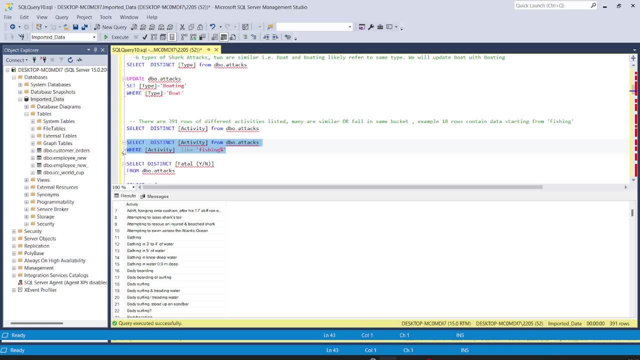 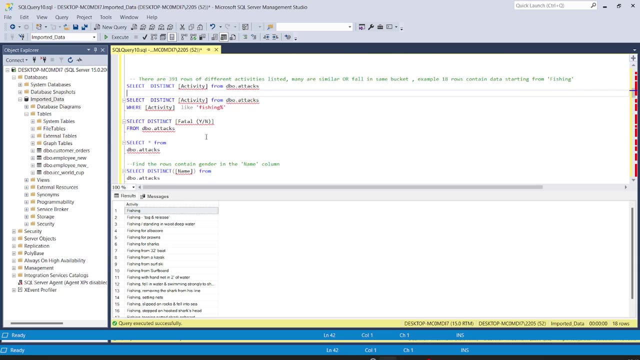 Okay, So we will check how many. how many activities are there which are similar or fall in same bucket? Okay, So we'll run this. So we have total 18 rows which contain the data starting from fishing. Then We will check for fatal as well, fatal column as well. 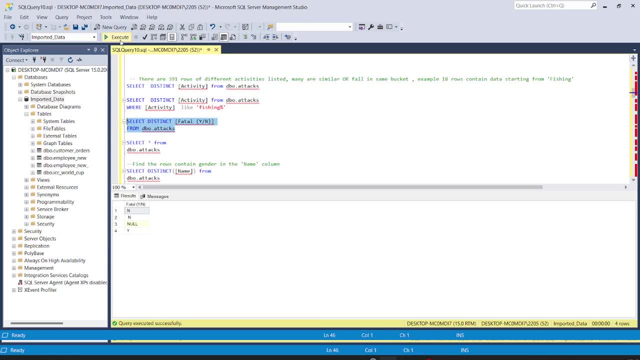 So let's run this. So we'll execute this. We have four types, So first and second is same, And the problem is, You know, here we have white space So we can update this. So for that what we will do, we will copy this query here. 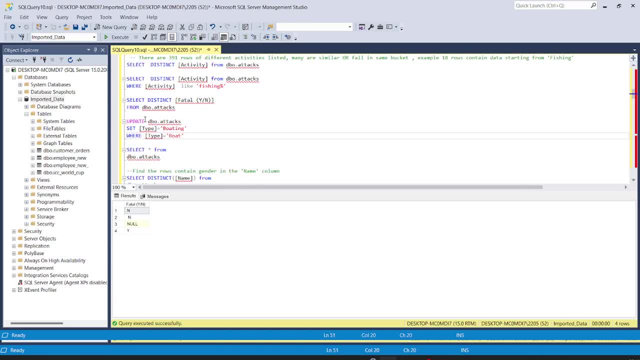 And what we can do. We will update the table, set This column fatal y, n. Okay, Is equal to n where this fatal column has space and value. Okay, So we need to update all those rows where we have space, and So let's run this. 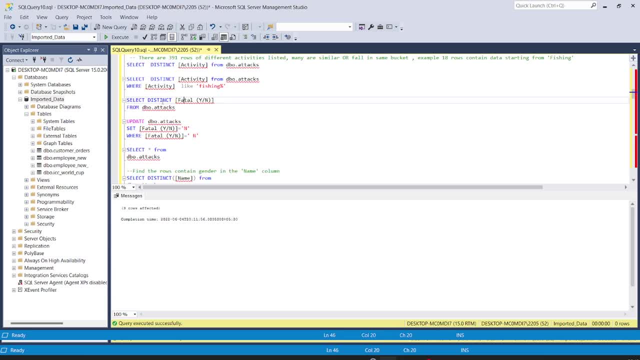 So you can see three rows are affected. Now, if we go back to this command, select distinct Fatal from DBO attack. Now you can see we have only three rows And none and one. Now we will check for Our name as well. 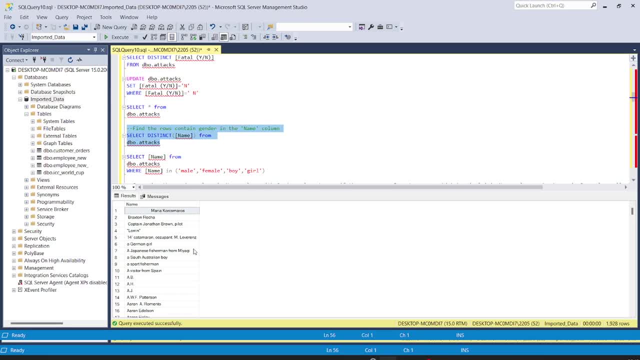 So select distinct name from attack. So here you can see, we have some rows which contain gender as well in the name column. So in order to find those rows, we will write this command: select name from the table- attacks. We are named in. 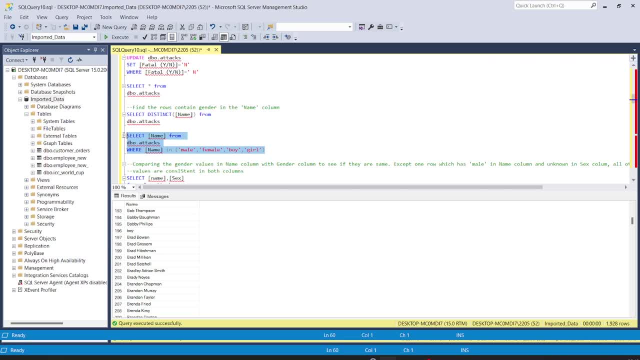 Male, Female, Boy, Girl. Okay, So we will run this code And now you can see we have total 126 rows here, Okay So? so now we will compare this gender value is named column with the actual gender column to see if they are same. 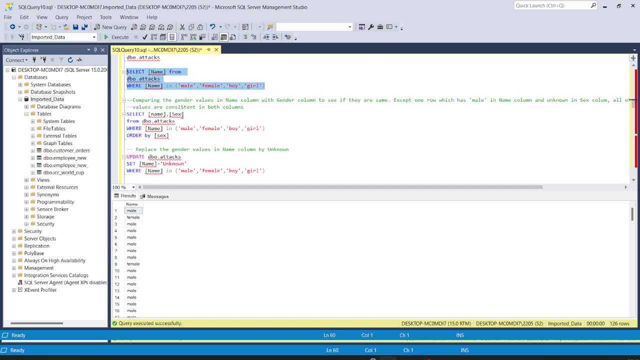 So we will write this command: select name and sex from attack table, where name in male, female, boy or girl order by sex. Okay, So we'll run this code And now you can see there is only one row which has male, but in sex it is none. 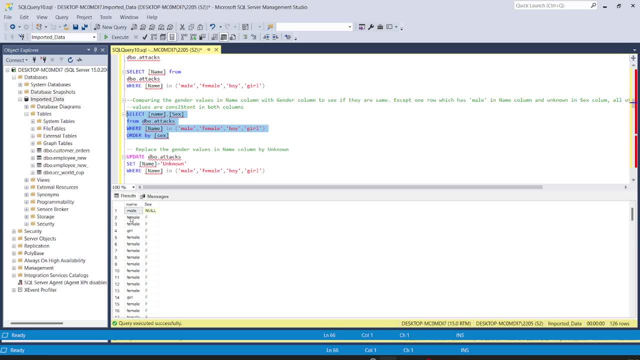 Okay, And in other rows it is matching like if we have female in name, then it is f in sex. So what we will do? we will replace the gender values in the name column with unknown where, where we have name in male, female, girl and boy. 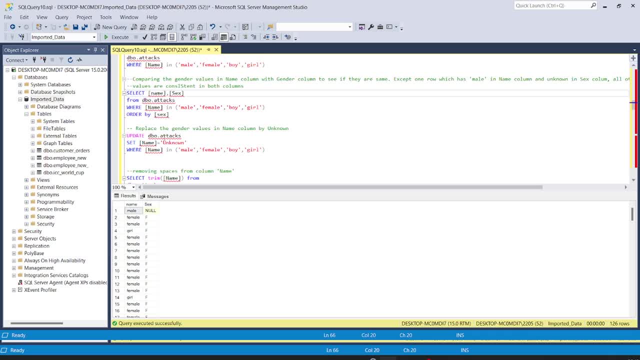 Okay, So for that command is: update table attacks. Set name is equal to unknown. where name in male, female, boy and girl. Okay, Let's run this code Now. it has affected 126 rows, So let's go. Let's run this query again. 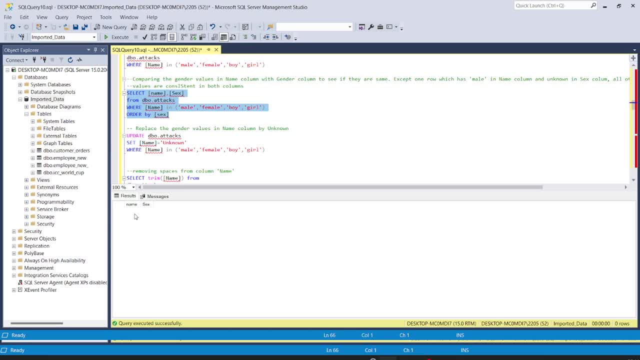 So now you can see that it has returned no results, because now we don't have any row where name in male, female, boy and girl. Okay, After that, in order to clean our data. So sometime in data We see some white space as well. 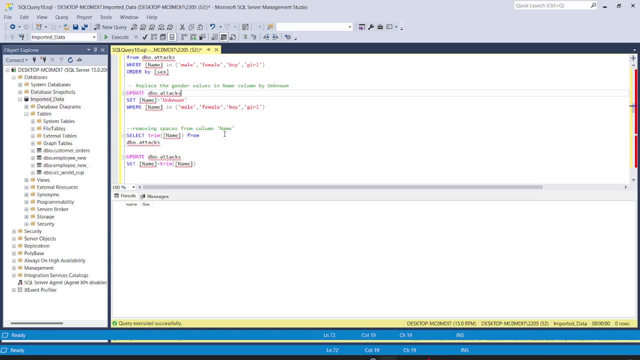 So, for example, in our name column we have some white space. So for that, what we will do, we will use trim with name column. Okay, So in order to update the table, what we will do? update table name attacks. Set name is equal to trim name. 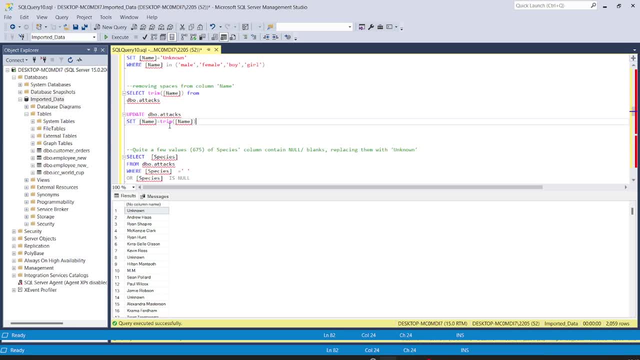 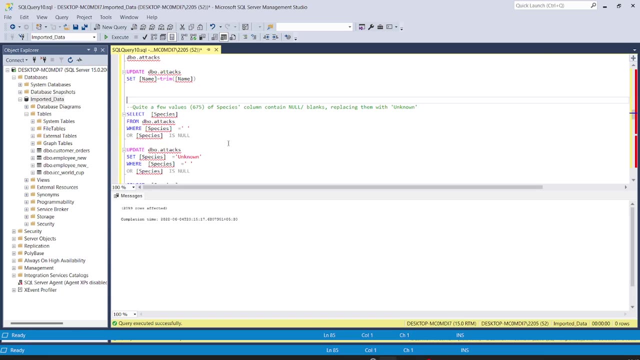 Okay, So we are using this trim function to trim our data, So to trim our value, So it will remove all the white space. So let's run this code Now. you can see 2059 rows are affected. Now we need to check the species column where species is null or where we have some white. 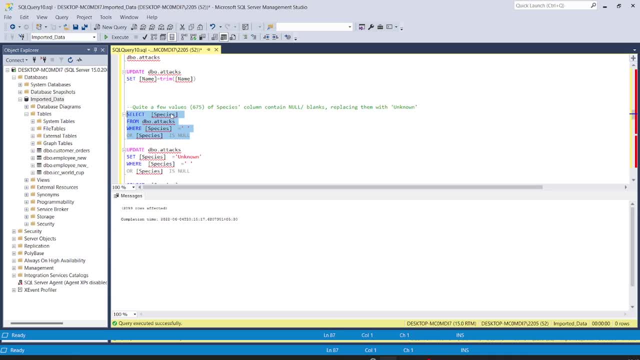 spaces. So we will run this query: select species from attacks table where species is equal to blank space or species is equal to null. Okay, So you can see we have total 672 rows where species is null. Okay, So we will update our species column with unknown, where species is null or we have white. 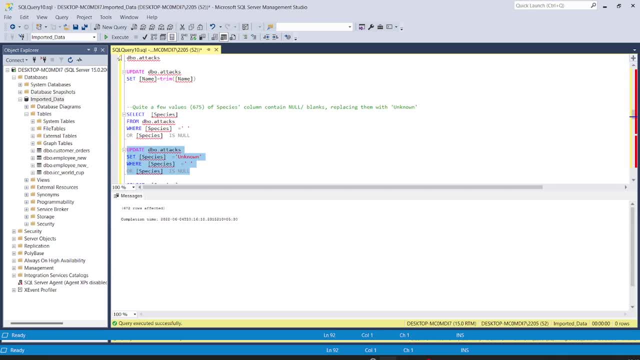 space. So we will run this command Now. 672 rows are affected. Okay, So let's check our data again. Select species from the viewer text. So now you can see we have some unknown values, Some unknown value as well where it was null before. 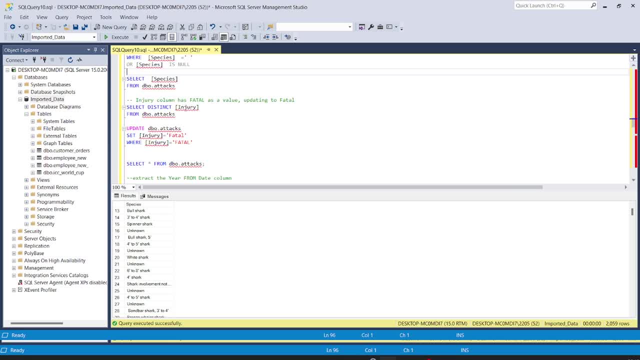 Okay, So now we will check our injury column, Select distinct injury from attacks. So we have total 1381 rows. Okay, And you can see, here we have this fatal value which is in capital letter, So we need to change it to camel case. 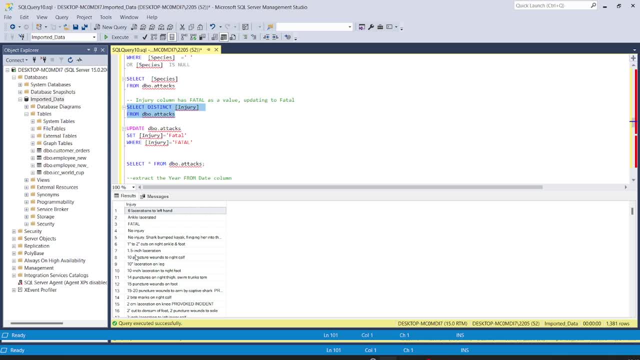 So for that we will update our column. Okay, So update the table Set. injury is equal to fatal, which is in camel case. where injury is fatal, which is in upper case. Okay, Let's run this code Now: 1351 rows are affected. 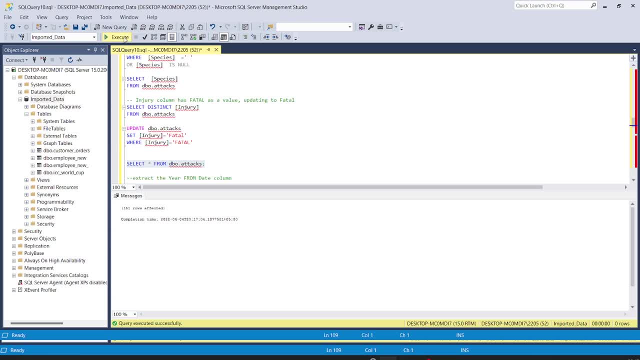 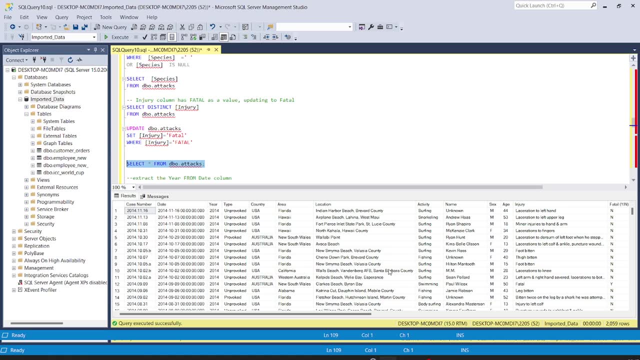 Okay, So let's check our data. So now you can see our data is looking in much better state, Like we have removed the null, We have removed the white spaces, We have transformed our data as well. Okay, So now we have the data as well. 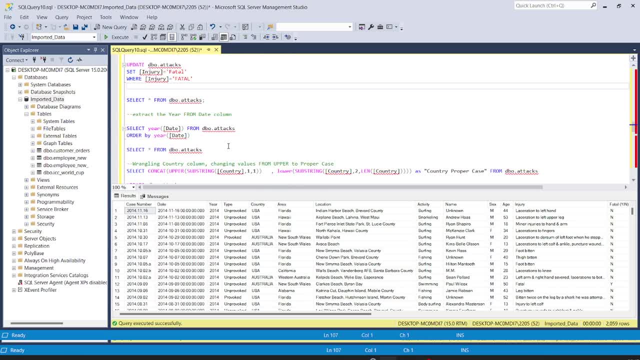 Like which was redundant. Okay, So now if we need to extract the year from the date column, as you can see the date column is in date format with timestamp, So for that we have this year function. So select year: We will use year function on date from attacks table and order by year. 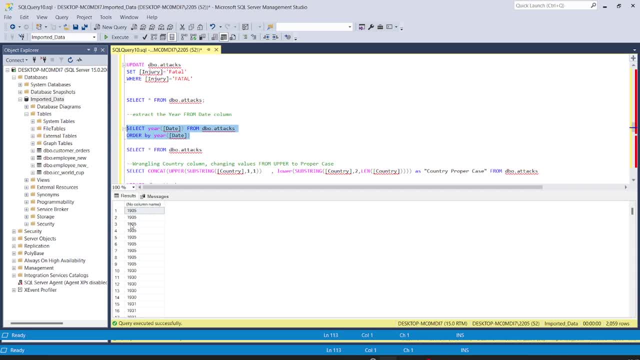 Okay, So let's run this. So now we have got year as well in ascending order, As well as the date column. As we have not defined it should be in ascending or descending, So by default it is taking it in ascending order. 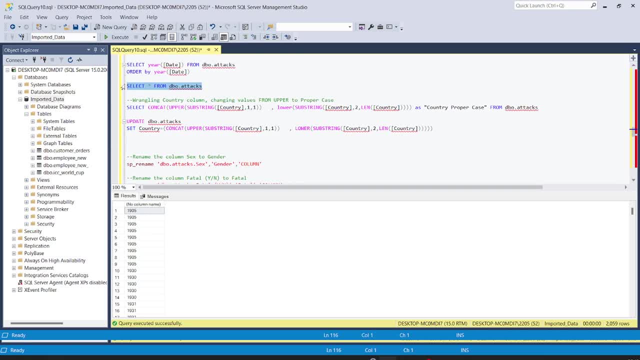 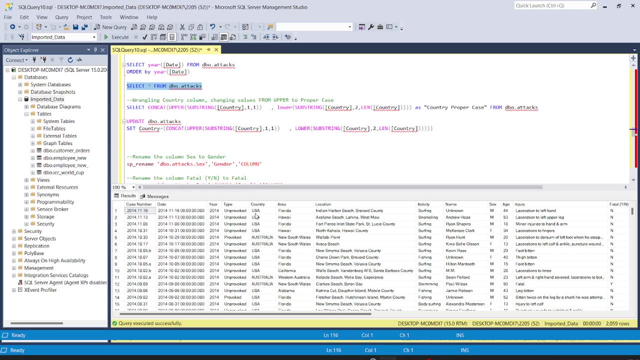 Okay, Now let's see our data again. So, as you can see, in country we have our values in capital letter, So let's convert it into the camel case. So for that, what we will do, we need first letter in capital letter and all other letter. 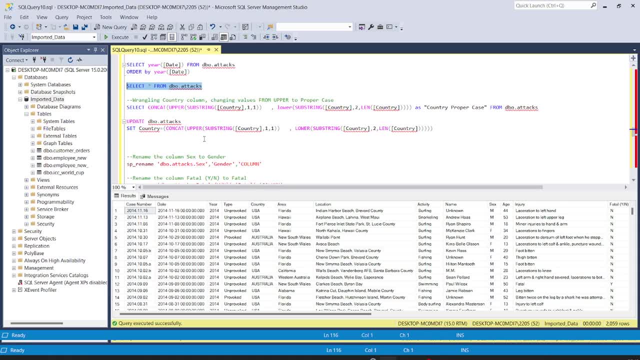 should be in lower case. So for that first, we will what we will use. We will use substring function and we will take only first value, Okay, And we will change that in upper case, Okay, And after that we will concat this value with our rest of the letters. 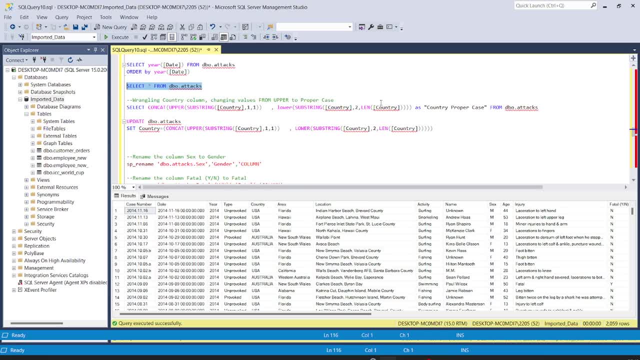 So for that, what we will do, we will use substring function and we will start it from two till to the length of the value in the column, and it should be in lower case. Okay, And we are concatenating it with the first value, which is in upper case, and we will give. 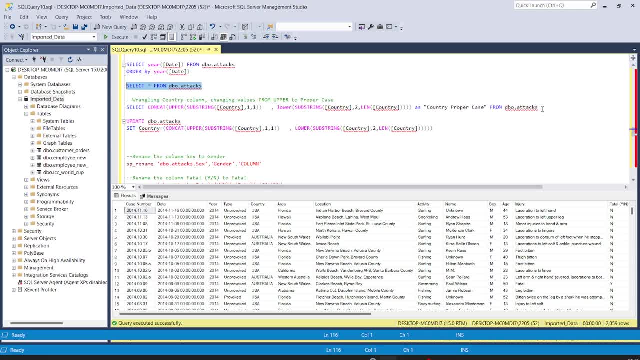 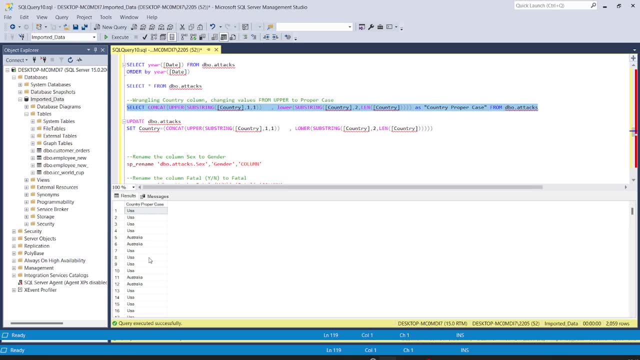 it in alias Country proper case from attacks table. Okay, So let's run this code. So now you can see we have a value in country column in camel case. So now we need to update the column. So right now we are just selecting and transforming this. 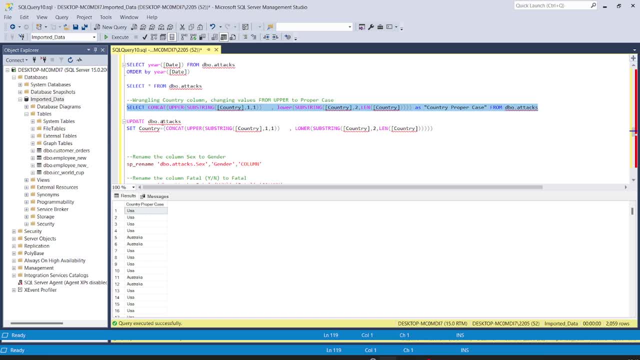 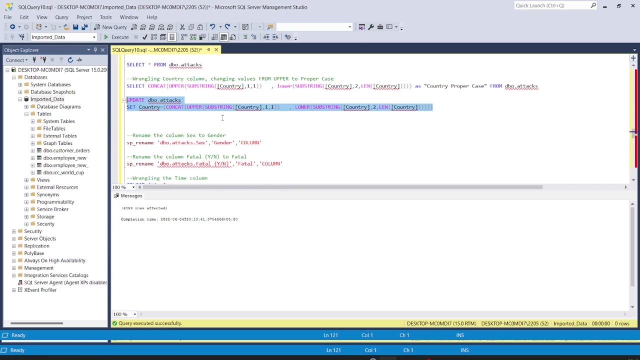 Now we need to update as well, So update attacks. table set country is equal to, and we will use the same logic here, So we will run this code. Okay, So 2015 rows are affected. Okay, So let's go to our data again. 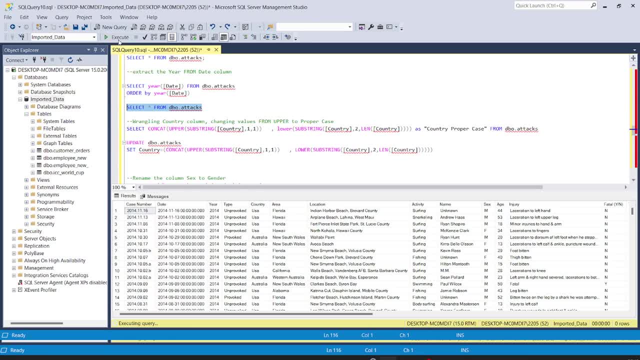 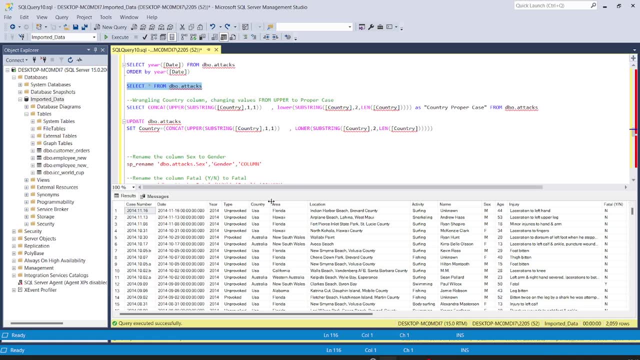 So now you can see we have country in camel case. Okay, So now we suppose we have this column sex. we want to rename it to gender. So for that we will write this command: SP rename. then we will mention the table name. 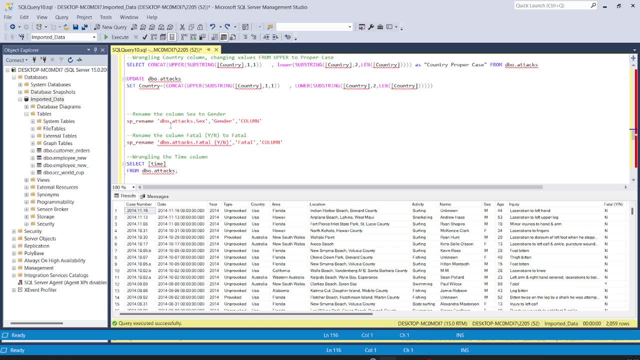 which is our attack dot sex and we need to rename this again. So we have this column sex, So we want to rename it gender. So for that we will write this command: SP, rename sex and we need to change it to gender. okay, let's run this quick. 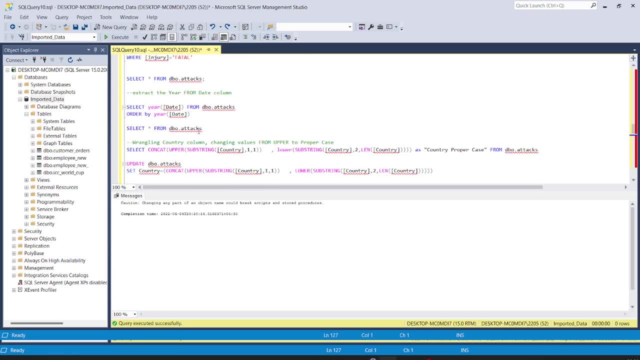 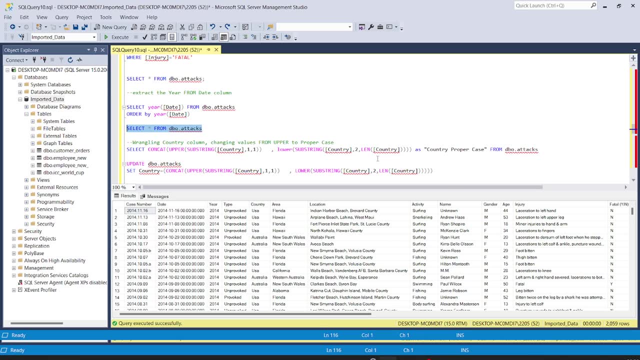 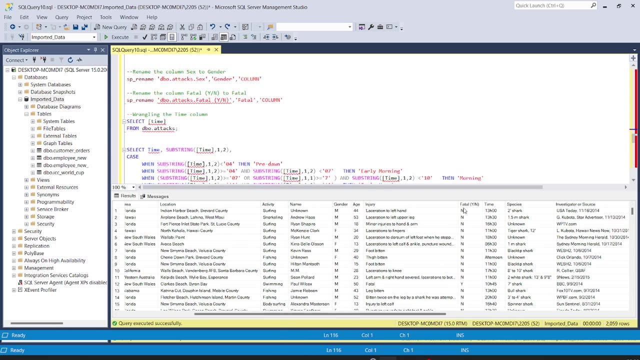 so it has renamed this column. so now if we check our data we can see here it has it has changed to gender. okay, now we will do the same thing to fatal column as well. so if we go to this fatal here we have uh in yes or no in brackets, so suppose we want to remove it? um, so again, we will write this: 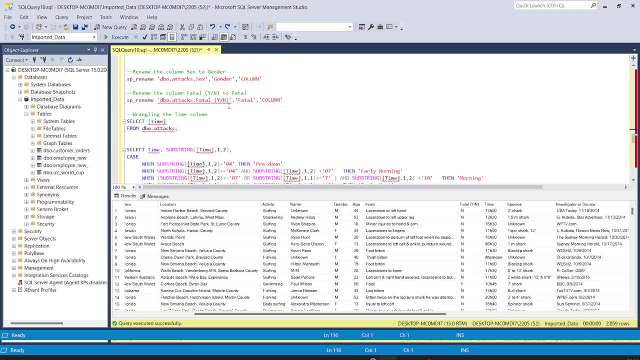 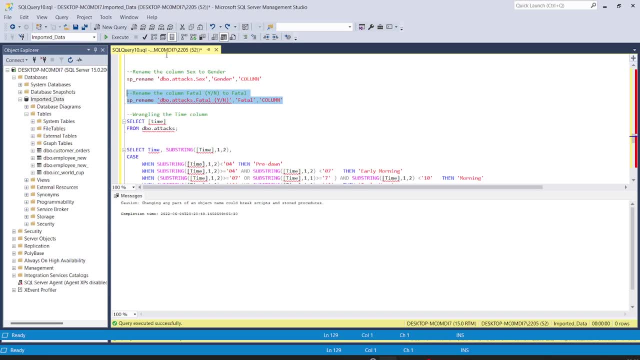 code sp rename and then column name is fatal yn and what we want here, fatal only. okay, so let's run this. so it has changed this as well. now let's check our time column in a text table so as you can see here, uh, we have this two digit number. 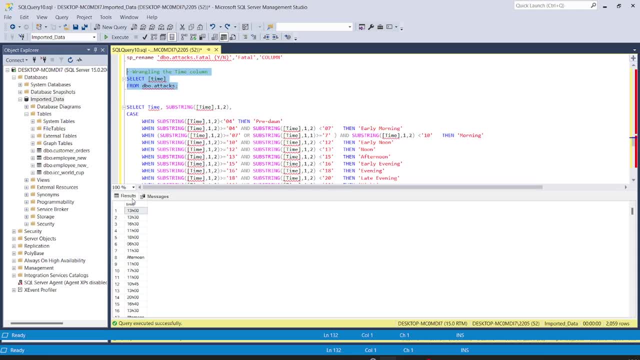 which shows us time like total hours. okay, so we have, uh, this in this format: 13 hour, zero, zero minute, and suppose we need to create one more column: attack time. okay, so for that, what we can do here, so we can write select, so we need time and we we need substring. so we need first two. 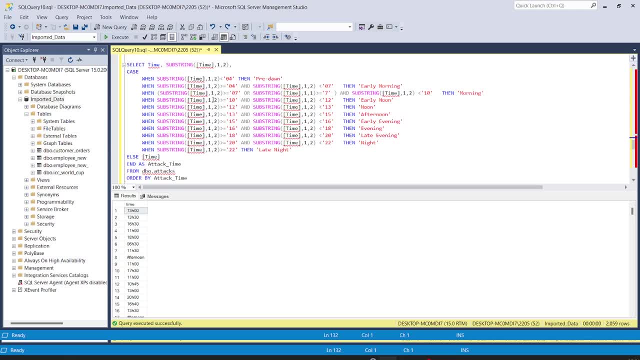 letter of time as well. okay, so what we will do? we will use the case condition here, case when substring time. so we need to take only two first two values, okay, so select so case when substring and two value first two values of time is less than four, then it should. then we need pre-dawn. 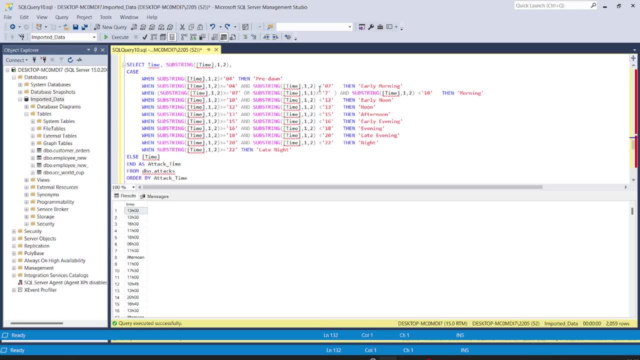 value, and if it is greater than four and less than seven, then it is early morning. if it is greater than equal to seven, or if it is, like in this format, seven and it is less than 10, then it should, and less than 12, then early morning. if it is greater than 12 and less than 13, it is noon. 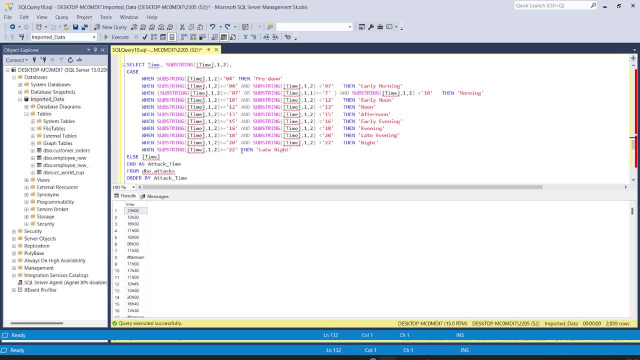 and similarly we will do for all other values as well. okay, and then we will end our case condition and we will give it an alias as attack time from attacks table and we are ordering it by attack time. okay, so let's run this. so now you can see we have got attack time as well. so currently we 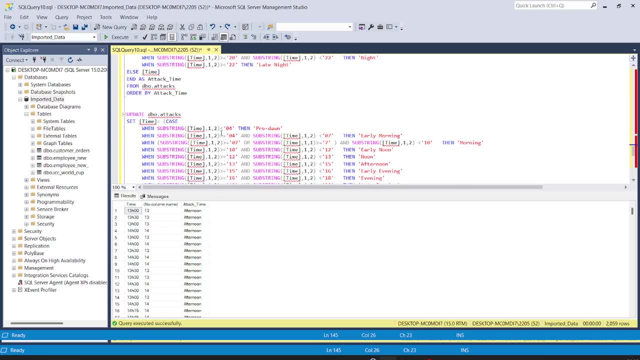 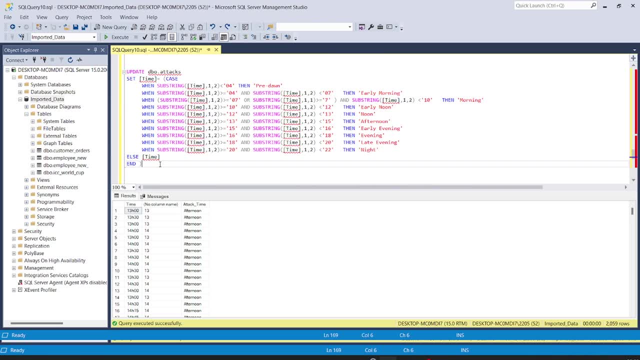 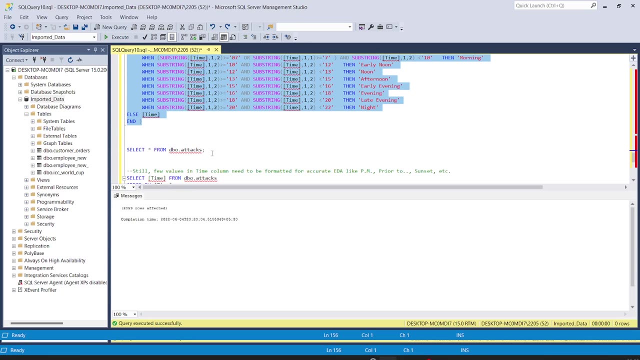 are just selecting and transforming this column, but now we need to update as well, so update attacks table and we need to set time, and then we will use the same logic here. okay, so we'll run this. so it has updated 2059 rows. okay, so let's run this code and check our data. select star from. 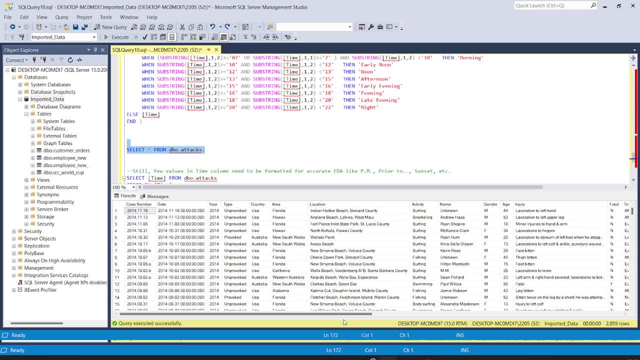 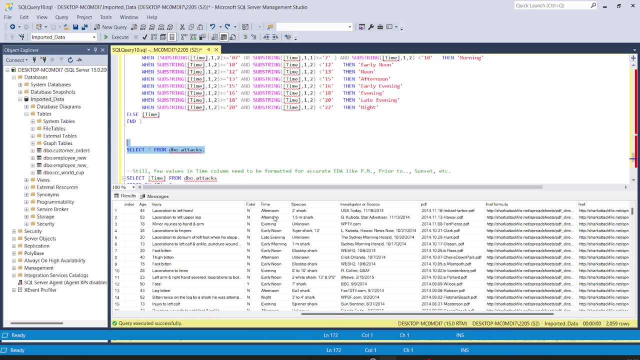 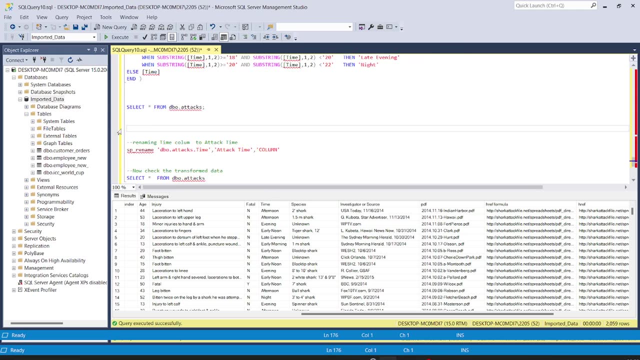 attacks table. so now if i go to the time column, so so now if i go to the time column, so now if i go to the time column, we can see here afternoon evening, early noon. so the data is in much presentable state now and we are getting meanings as well. okay, so now suppose we want to rename this time column to 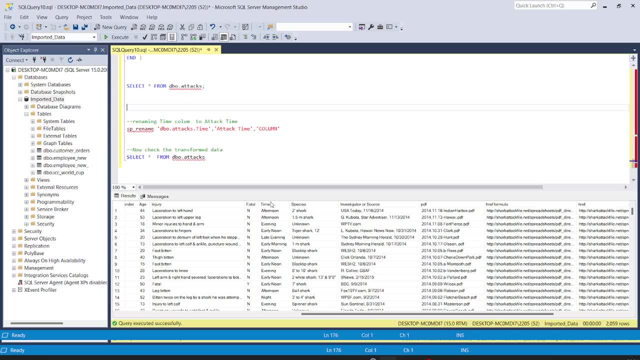 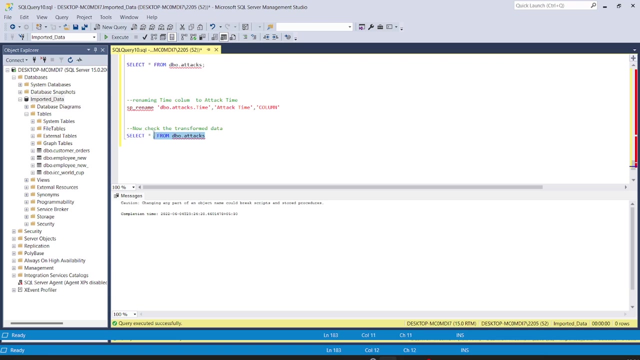 attack time as it shows at what time the attack has happened. okay, so for that again, we will run the same query, sp rename. then the column name is dboattackstime and we need attack time instead of time. okay, so we'll run this code. okay, so this has changed time to attack time. now we will check our transform data.